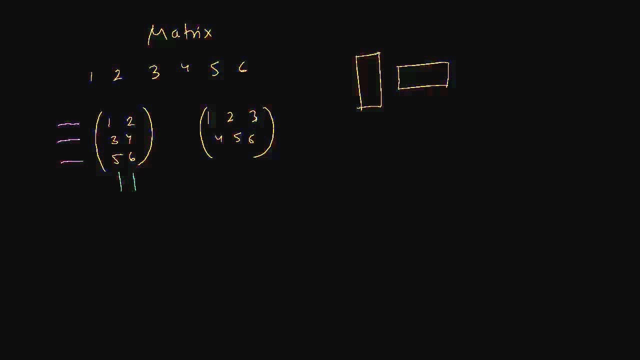 And the columns are 1, 2. And here it has 3. Two rows: 1, 2, and it has two columns, three columns: 1, 2, 3.. The size of a matrix is written as first we write the row, So 3 here by 2 here. So we say it's a 3 by 2 matrix. 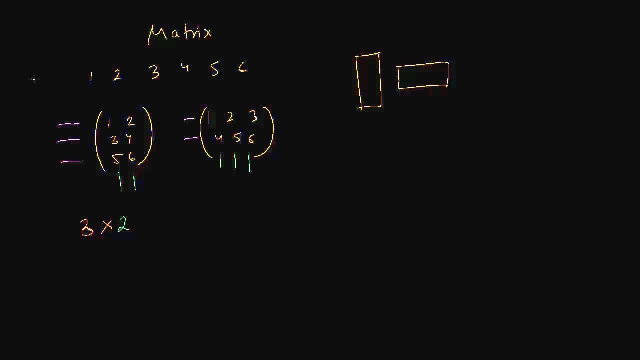 And here we have 2 row times, 2.. 3 row, 3 columns, that's it. So when we have a matrix, it's all about the arrangement, And the arrangement is mentioned that it is number of rows with the number of columns. 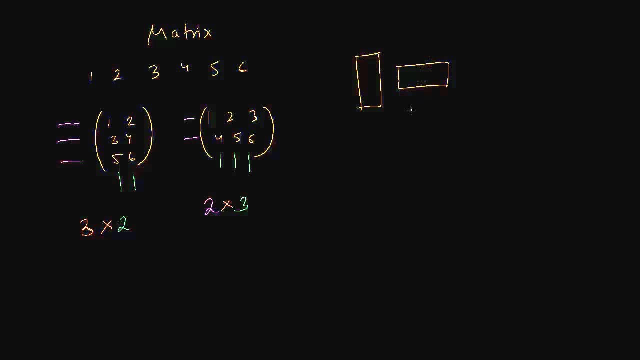 So let me write it here. So the size of a matrix is row by column And it is written as a number times another number. We don't multiply it, we just call it times. When we have these matrices, it is possible to have a square matrix. 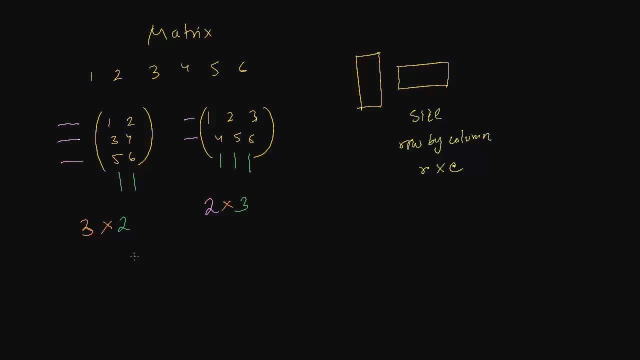 A square matrix is simply where the number of rows and the number of columns are equal. So this can be 1,, 2,, 3, 4.. So here we have two rows and we have two columns. So this is a 2 by 2 square matrix. 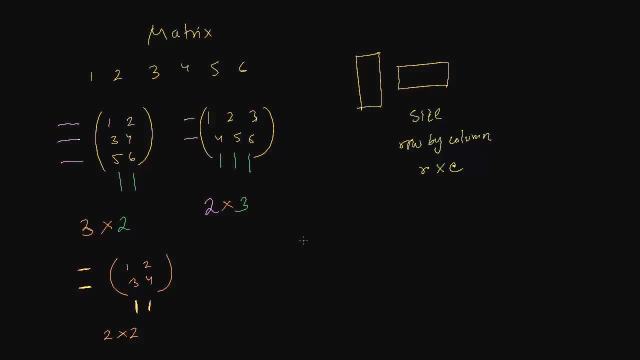 The important thing about matrix is the number of rows. The important thing about matrix is the number of columns, The arithmetic operations. So the arithmetic operations are addition and subtraction. So it's fairly simple. Let me show you how this is done. Addition is: let's write down the matrix. 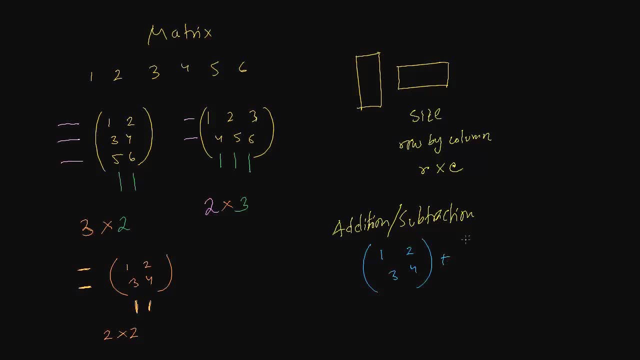 1,, 2,, 3, 4. plus we have another matrix, 5,, 6,, 7, 8.. So both are 2 by 2 matrices. It is important that the sizes of the matrix are the same. 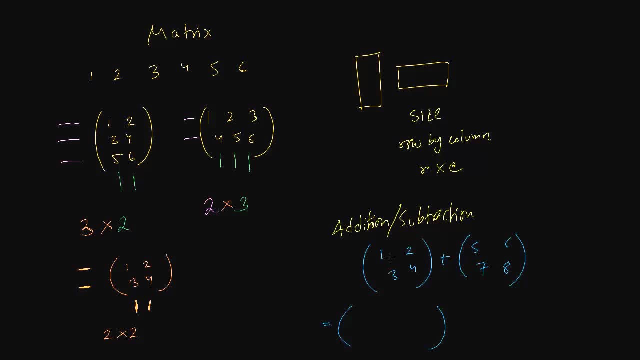 So addition is fairly simple. We just add up the same positions: 1 plus 5 is 6.. 2 plus 6 is 8.. 3 plus 7 is 10.. 4 plus 8 is 12.. That's it. 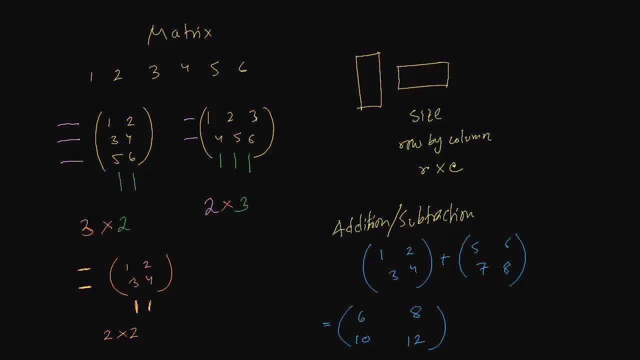 That's all there is to it. Subtraction works in a similar way. So when we have subtraction 1,, 2, 3, 4 minus 5,, 6,, 7, 8. So the subtraction works. 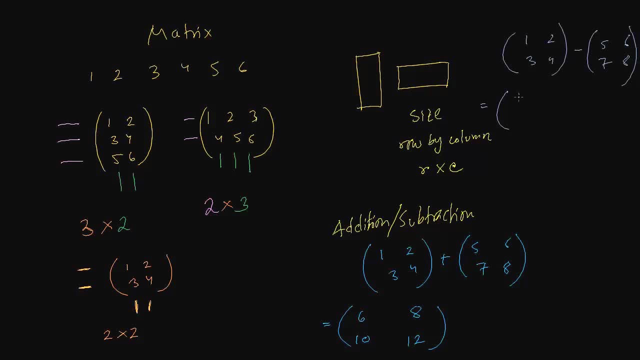 You just subtract the individual positions: 1 minus 5 is minus 4.. 2 minus 6 is minus 4.. 3. 3 minus 7 is minus 4.. And 4 minus 8 is minus 4.. 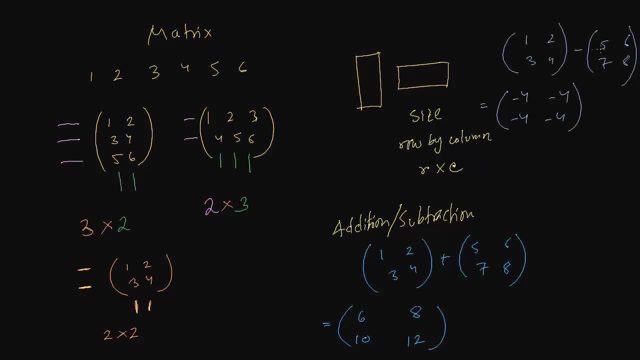 Subtraction. The individual positions are like that Subtraction. Another idea is Scalar Product. Scalar Product, Scalar Product, is multiplying the matrix with a single number. So if you want to multiply a matrix with 3.. 1,, 2,, 3,, 4.. 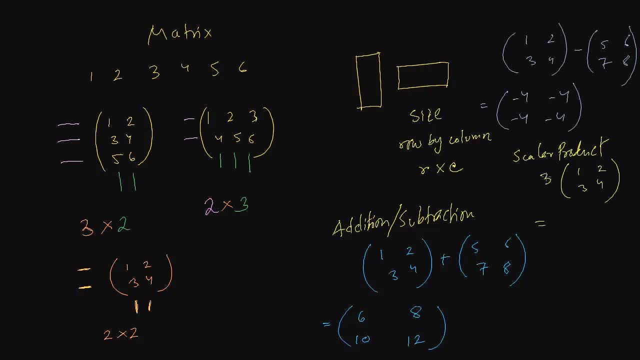 You want to multiply this matrix with a scalar product, It has to be 3x1, 3. 3x2, 6. 3x3, 9, 3x4, 12. is the scalar product? It doesn't matter. in case of scalar products, it doesn't really. 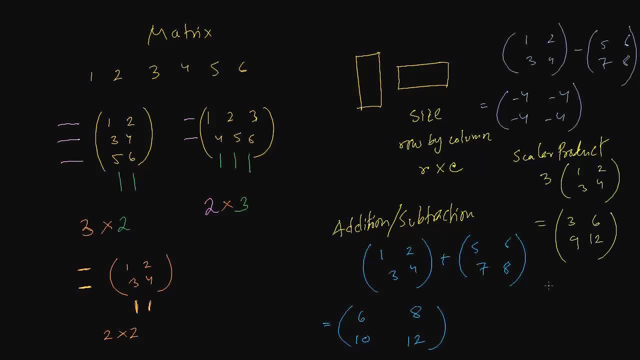 matter what the size of the matrix is. If I want to multiply 2 with 1,, 2,, 3,, 4,, 5, 6, so this is a 3 by 2 matrix, 3 rows and 2 columns, then it would turn out to be 2 into 1 is 2,. 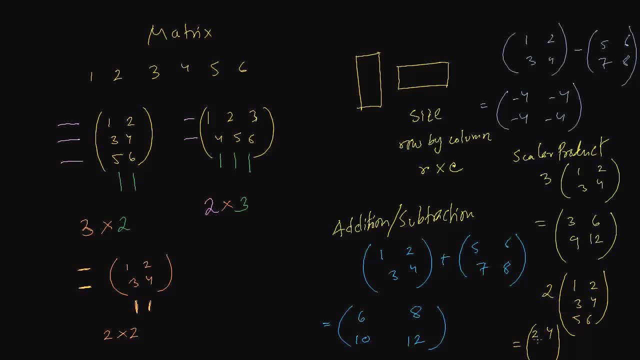 2 into 2 is 4,, 2 into 3 is 6,, 2 times 4 is 8, 2 times 5 is 10,, 2 times 6 is 12.. So that is the scalar product. Now, a more challenging arithmetic operation, apart from addition and 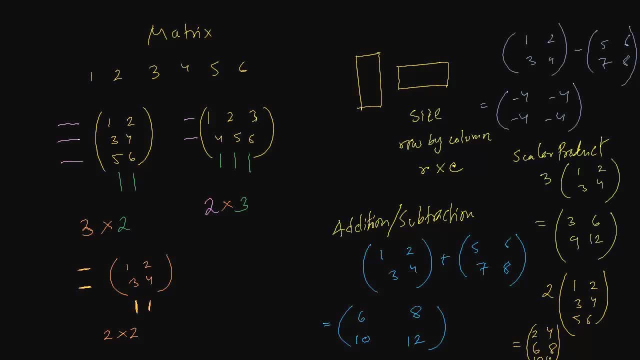 subtraction is fairly simple. It's the multiplication of matrices, which is not as straightforward as it might seem. what addition and subtraction is? So this is what it is. So if you want to multiply 2 matrices, multiplying matrices- So if you have 1,, 2,, 3,, 4 and you want to multiply this with 5,, 6,, 7,, 8, so this is what is done. 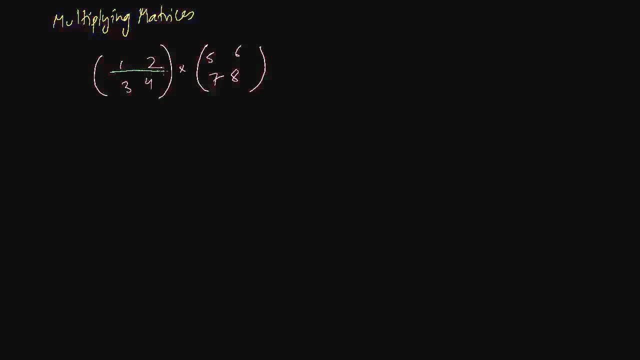 First the row is taken here. this row is taken and with this we multiply this column. The first reaction might be: since we add the same position, 1 plus 5,, 2 plus 6,, 3 plus 7,, 4 plus 8, this is not what's happening. This is a bit different. It's more complicated. So the obvious thing might be it should be 1,, 2,, 3,, 4,, 5,, 6,, 7,, 8, and here's the first one. This is not what's happening. This is a bit different, It's more complicated. So the obvious thing might be it should. 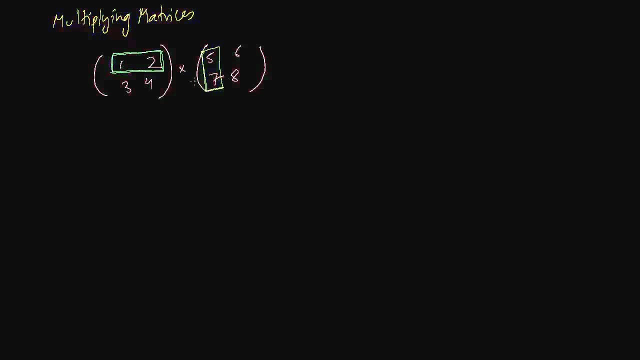 be 1 x 5,, 2 x 6,, 3 x 7,, 4 x 8, but this is not happening. So what is happening? The first row is taken and it is multiplied with the first column of the second matrix, When this: 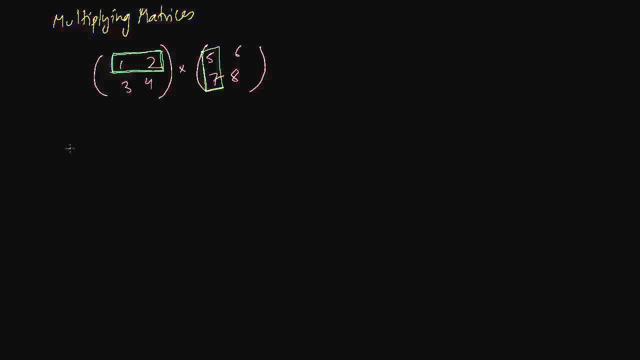 is done, we get something like: 1 x 5 is going to give us 5, plus 2 x 7 is going to give us 14.. So what we are doing here, we are multiplying this 1 with this. So this is the product, and. 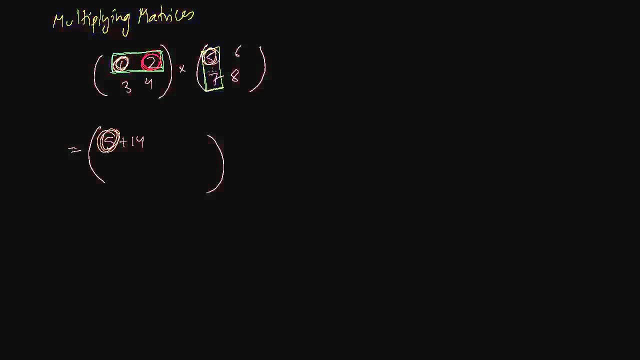 then we are multiplying this 2 with this 7.. So this is the product. So this is what we are doing. So the next thing that we have to do after that is that we multiply this same row with the next column. Then it turns out to be: 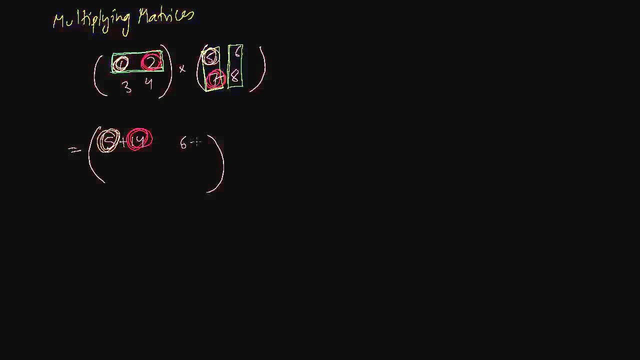 1 times 6 is 6, plus 2 times 8 is 16.. And we proceed to the next one. So the next row here is 3, 4.. So when we do this, it becomes: 3 times 5 is 15, plus 4 times 7 is 28.. 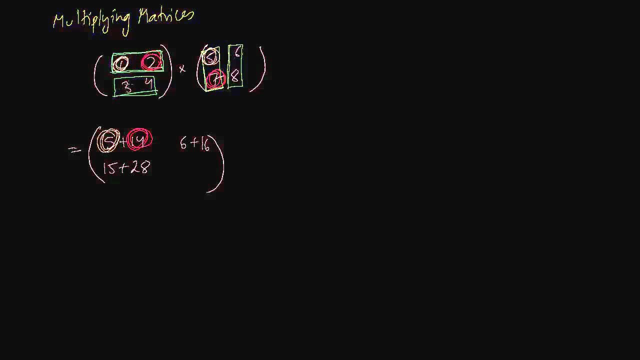 Then we move on to the next column, which is: 3 times 6 is 18 plus 4 times 8 is 32.. And we simply add it. So 5 plus 14 is 19.. 6 plus 16 is 22.. 15 plus 28 is 43.. And 18 plus 32 is 41.. 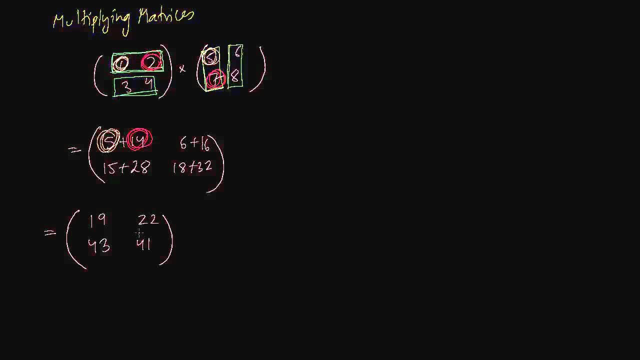 So that's the addition. This should be 50. This should be 50. So 4 plus yes, So that's the addition and we add it, And that is the multiplication of two matrices. Now, the multiplication of two matrices doesn't mean it has to be of the same size. only It can be of different, because every multiplication is not allowed. 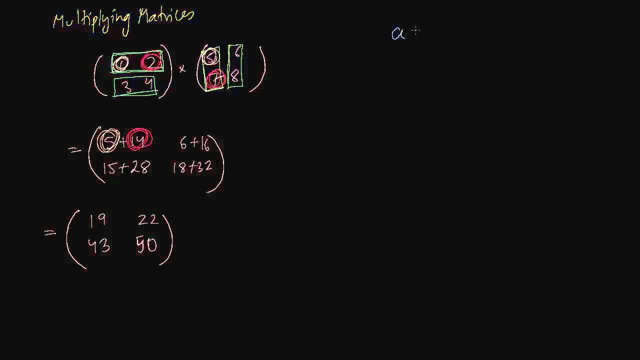 What happens here really is the first of this Suppose. this is the size of the first matrix, And the size of the second matrix is this: B times C. You can multiply two matrices only if this thing and this thing matches. That means these are the possible multiplications that are allowed: 2 times 3, 3 times 1, or 3 times 1, 1 times 2.. 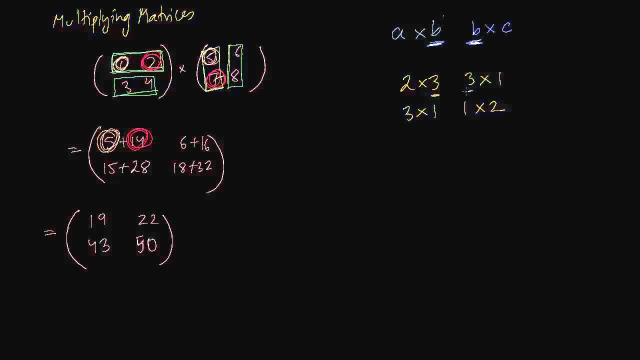 It doesn't really matter what the other, But this and this they have to match. So if you take a look at, if I give you two examples, The first one is 2 times 3.. So 2 rows, 3 columns. 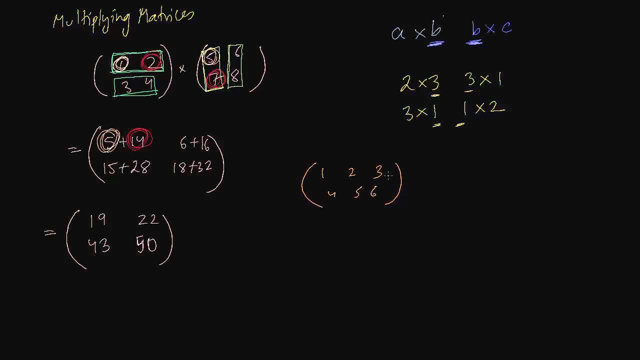 So 1, 2,, 3,, 4,, 5,, 6. Multiplied by- we often don't write this multiplication simply, We just write this bracket. This would be 3 rows, 1 column. So let me write 7,, 8,, 9.. So it has 3 rows and 1 column. 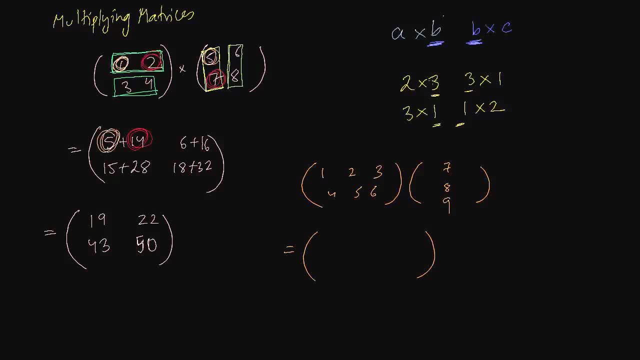 This multiplication is, of course, allowed. Because it's not allowed? Because this column of the first matrix matches with the number of rows of the second matrix, So that makes it. So we are going to multiply this row one more time with this column over here. 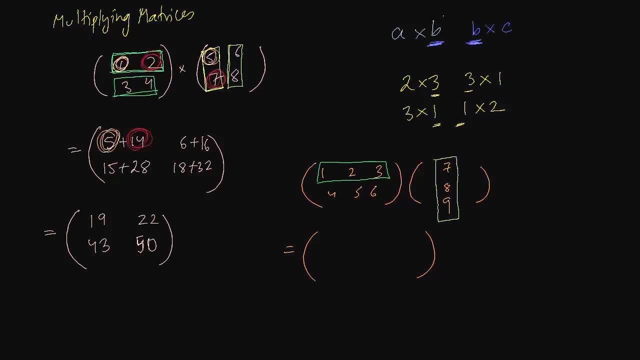 So we have to do this multiplication, So let's move on with this. So 1 times 7 is 7.. Plus 2 times 8 is 16.. Plus 3 times 9 is 27.. Next we have the next row over here, which is 4,, 5, 6.. 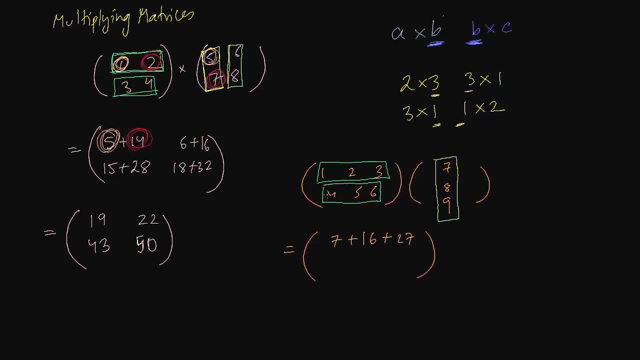 And when we multiply that we get: 4 times 7 is 28.. Plus 5 times 8 is 40.. Plus 6 times 9 is 54.. Yes, So this is what we get If we add this now. I am going to use a calculator now. 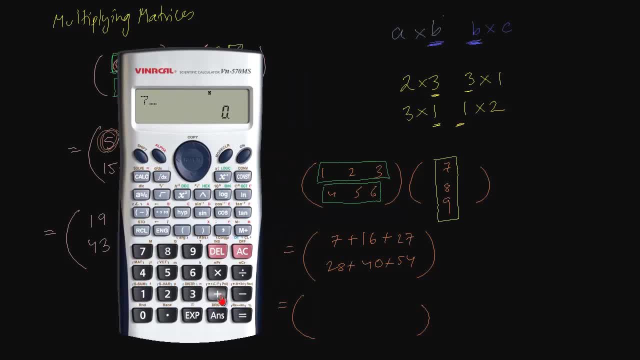 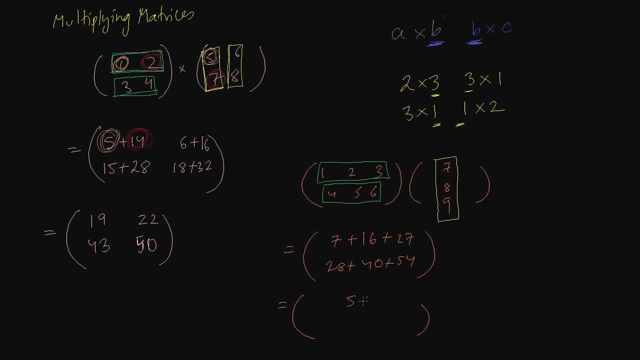 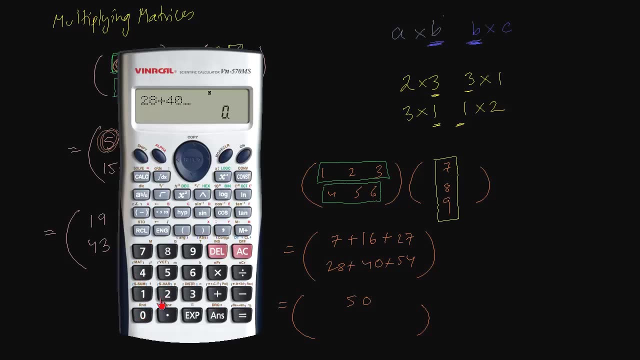 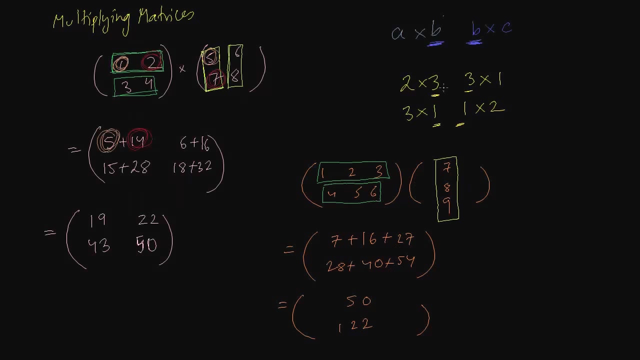 We are going to get? We are going to get 7 plus 16 plus 27.. This is 50. And 28 plus 40 is 68. Plus 54. This is going to be 122.. Now, if you notice, this is 2 by 1.. 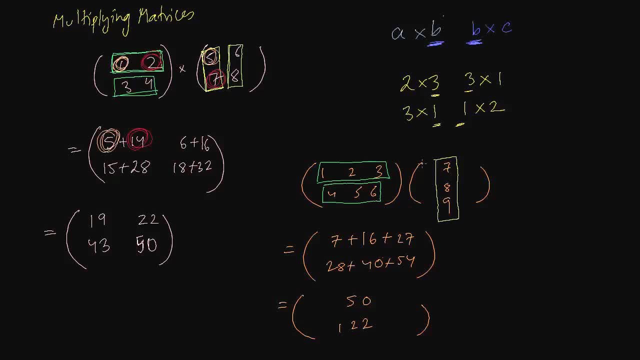 And the size of this matrix is 2 rows and 1 column, 2 by 1.. That means we can safely say that whatever is left over, that is the size of the remaining matrix, 2 by 1.. So the size of this matrix is going to be 3 by 2.. 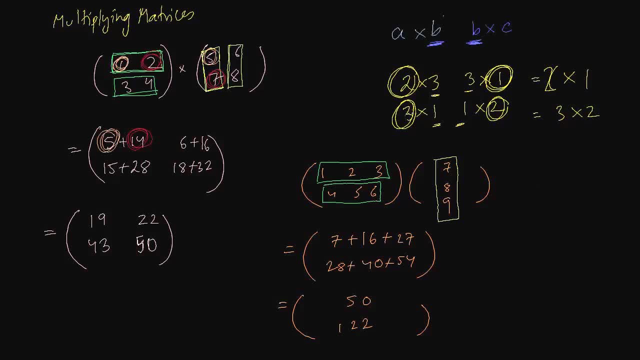 So let's do another example with this type of sum: If we have a 3 by 1 matrix, that is going to be 3 rows and 1 column, So 1, 2, 3.. 3 rows and 1 column. 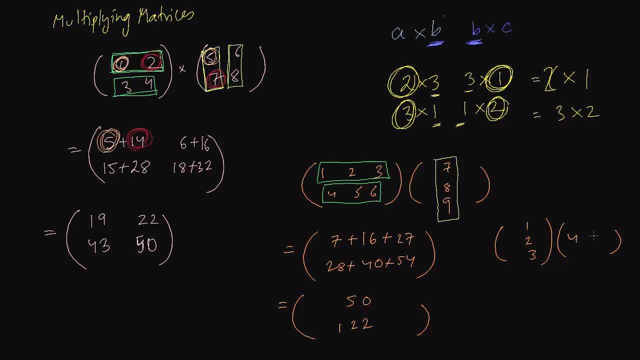 We have 1 by 2.. So 1 row, 2 columns, So 4, 5.. So can we multiply this? Of course, Because this thing and this thing matches, So it is allowed that we can multiply this. 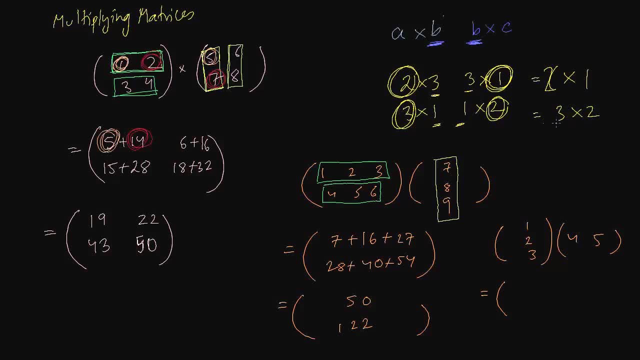 And the product is going to be 3 rows. That means 1, 2, 3.. And 2 columns 1, 2.. So that is going to be the product. So let's check whether this is the case indeed or not. 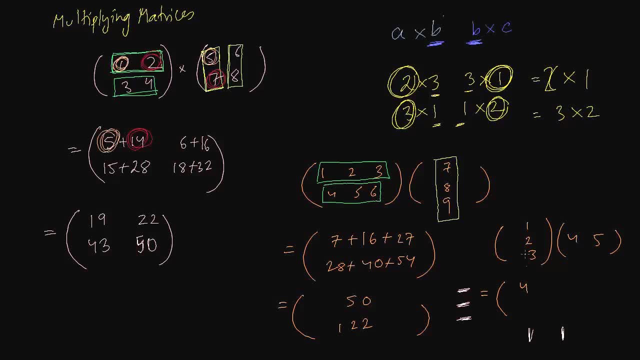 So 1 times 4 is 4.. The next one. So this is the first row. The first row contains only one element, And this is the first column. We multiply that, And this is the second column. That is what is happening. 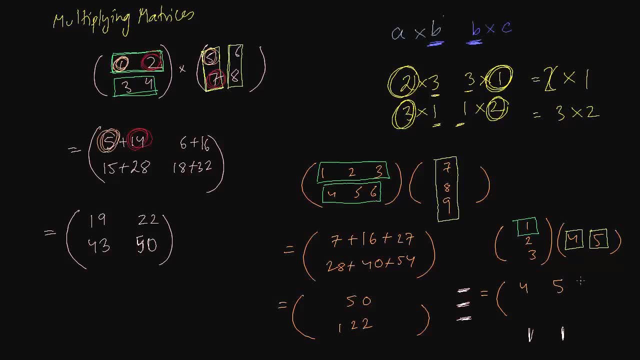 So that turns out to be: 1 times 5 is 5.. So we got our two columns now. Now the second row, So 2.. So 2 is going to be: 2 multiplied by 4 is 8.. So we get 8 here. 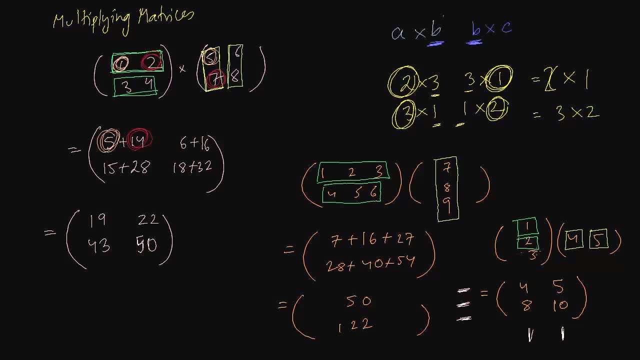 And 2 multiplied by 5 is 10.. Now we have the third row to think about. So this is the third row, And it turns out to be: 3 times 4 is 12. And 3 times 5 is 15.. 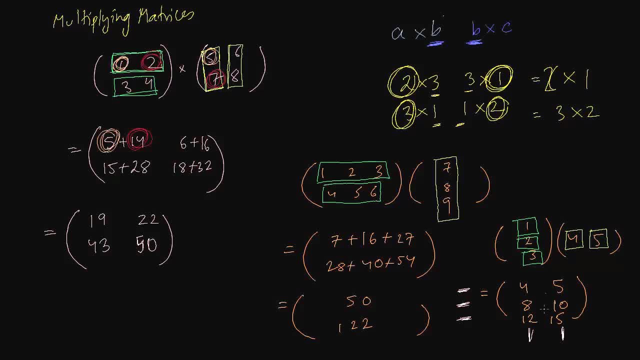 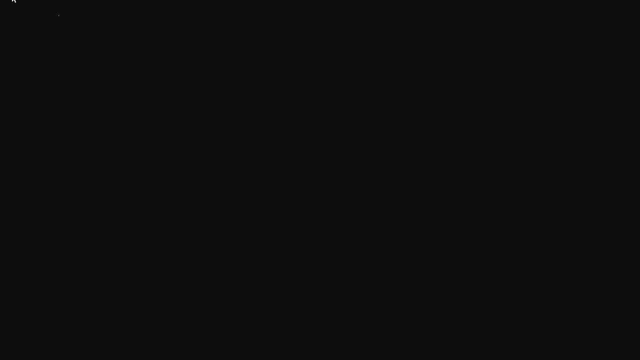 So we have a product which is 3 rows and 2 columns. There is a special bunch of matrices known as 2 by 2 matrices, So 2 by 2 matrices, 2 by 2 matrices, Which is the plural of matrix. 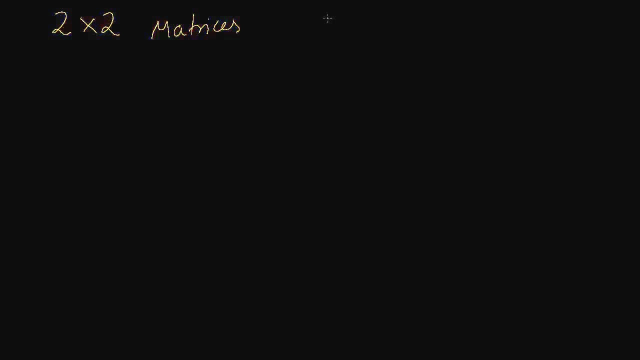 So if it is 2 by 2. That means the number of rows equals the number of columns, That is a square matrix. So 2 by 2 matrix is a square matrix here. So the first thing that we have to do 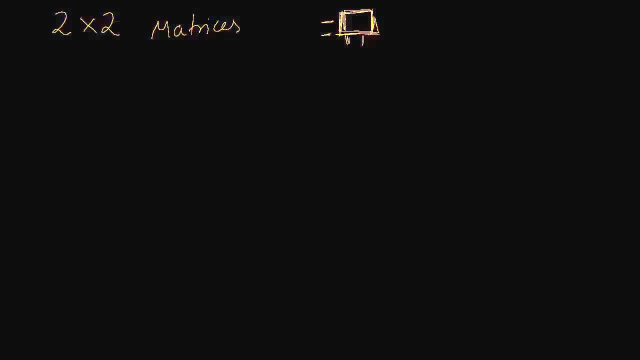 The first thing that we have to know is the determinant of a 2 by 2 matrix. The determinant of a 2 by 2 matrix is a special number. So the determinant is a special number with which we can use other stuff. We can solve systems of linear equations and things like that. 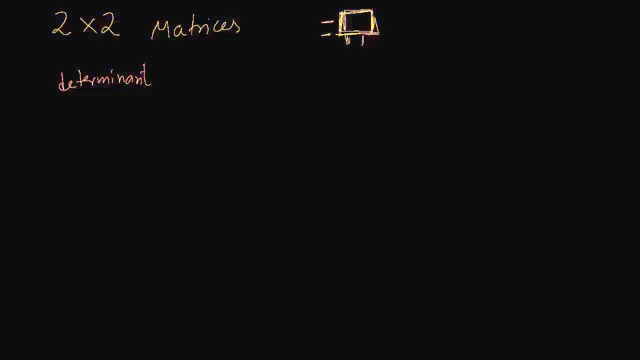 So if you have a 2 by 2 matrix like this, I am writing the algebraic version- A, B, C, D, And if you want to find the determinant of that, You just simply write it with vertical bars over here. 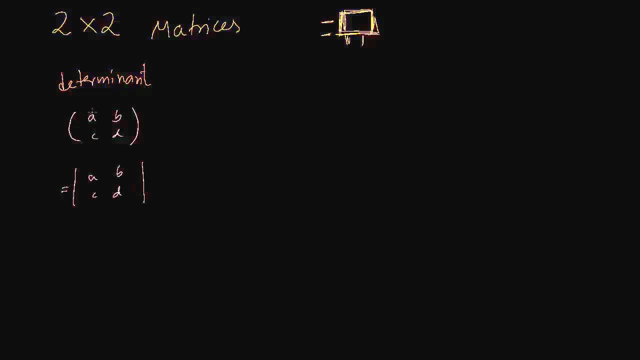 You write A, B, C, D. So this is a matrix, An arrangement of numbers, And this is this 2 bar signs over here. It means you are finding the determinant of that matrix And that determinant is a special number which we multiply this A with D. 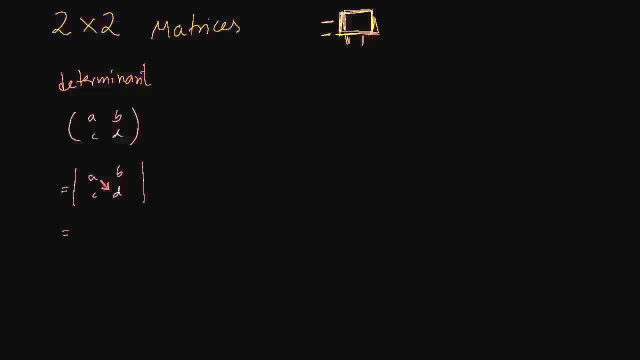 So we multiply this A with D, And we multiply this B with C And we subtract the 2. That's all we do. So it is going to be AD minus BC. That's the determinant of a matrix. So let me write here: 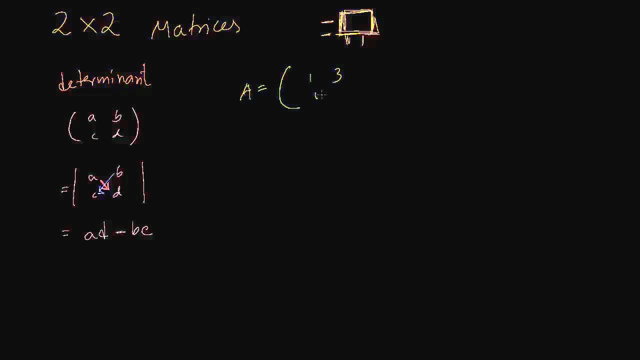 If you have a matrix 1,, 3,, 4,, 5. And they ask for this bar thing here, So you want to find the determinant of that matrix. That would be: 1 times 5 is 5.. Minus 4 times 3 is 12.. 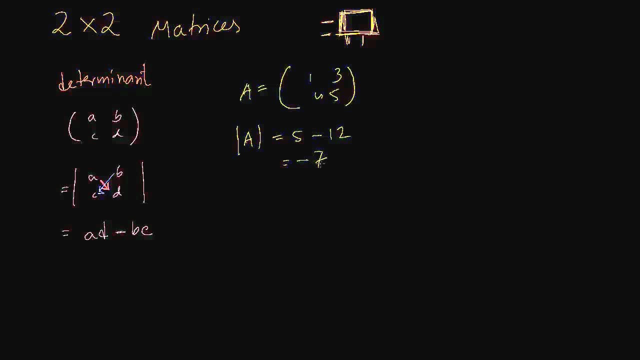 And the determinant is minus 7.. That's what we get Now if the determinant of a matrix is 0. This can happen if each and every term is same, Or it can also happen in other situations. If you have a matrix like this: 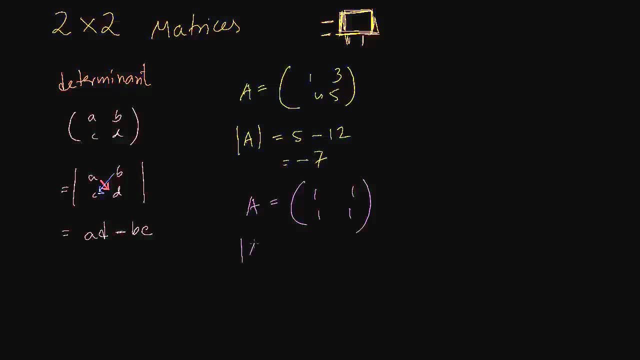 1, 1, 1, 1.. So what happens? The determinant becomes 0.. Because 1 times 1 is 1.. Minus 1 times 1 is 1.. 1 minus 1 is 0.. 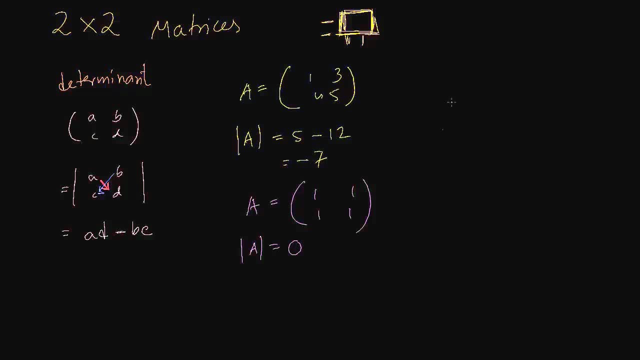 And it doesn't mean that all the elements have to be the same. It could be also different. For example, if you have a matrix 2,, 6,, 1, 3.. We know that the determinant is again going to be 0. 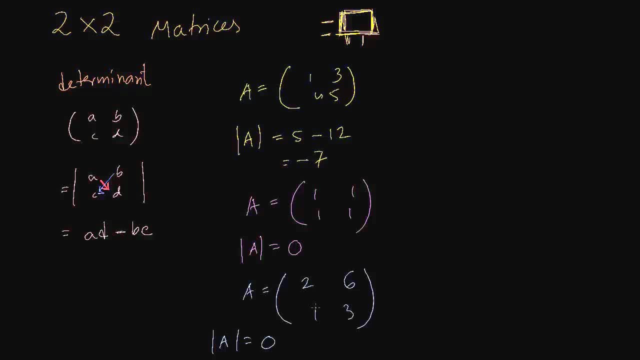 Because 2 times 3 is 6.. 6 times 1 is also 6.. There can be many different types of 2 by 2 matrices where the determinant is 0. Whenever a determinant is 0. We call that matrix a singular matrix. 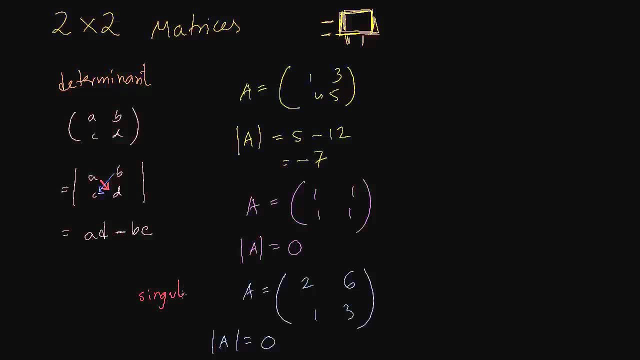 So we call that a singular matrix. Remember, first of all, it has to be a 2 by 2 matrix For it to be a singular matrix, And if it's not a 2 by 2 matrix, You cannot find the determinant. 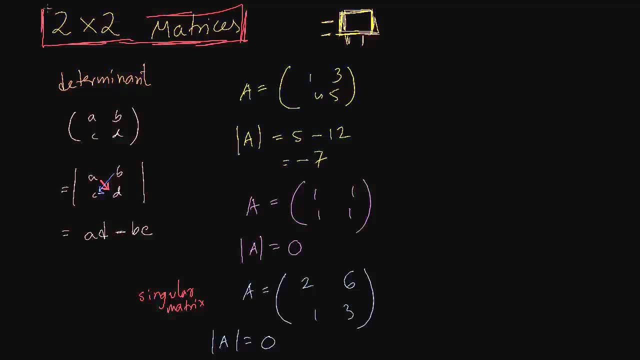 So the special rule is the 2 by 2 matrix. here The next thing that we have to find out is the inverse of a matrix. Inverse of a matrix. Now, you cannot invert every single matrix. It is important to remember: singular matrices has no inverse. 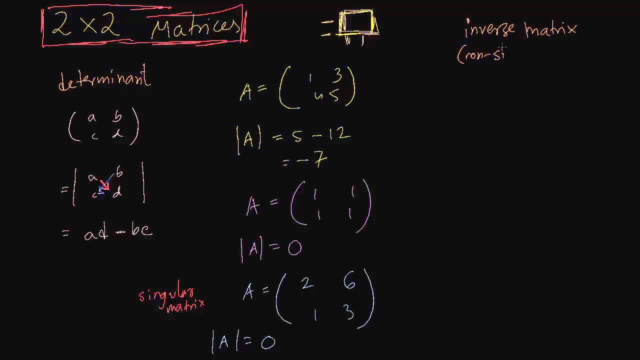 You can only inverse non-singular matrices. Okay, So this is how it works. If you want to find the inverse of a matrix, Suppose you have A, B, C, D And you want to find the inverse, And the symbol here is: 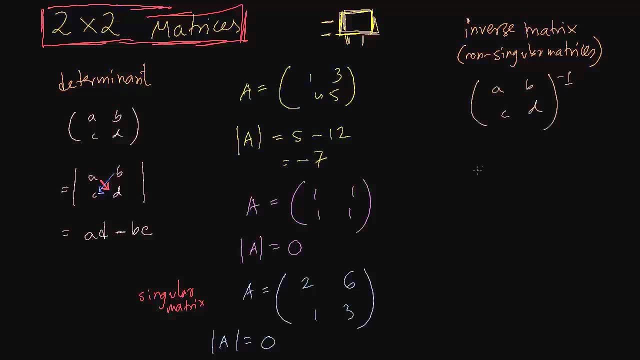 You put a little minus 1 over here. That means the inverse of a matrix. In determinant we put 2 bars And inverse of a matrix: we put a little minus 1 over here. So the rule is this: You take the reciprocal of the determinant. 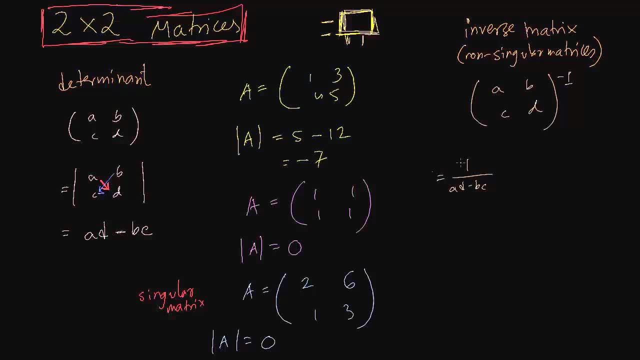 AD minus DC. Now that you see, if it is 0. We cannot divide a number with 0. That is undefined. It's a huge number. So that's why, if it's 0. If it's a singular matrix, We cannot have the inverse of that matrix. 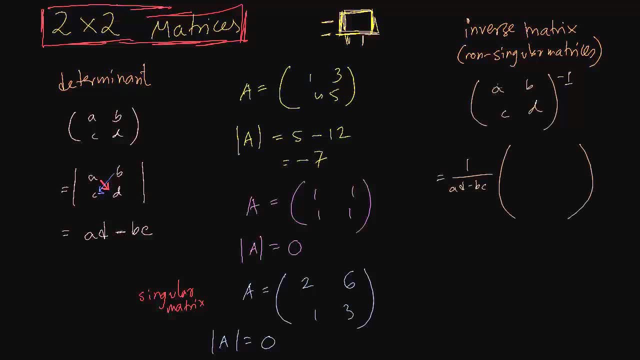 And the rest is just a trick. You change the positions of these diagonals, You put the D over here And the A over here, And then you change the signs- Plus, minus signs- of these. So these are both positive, You make it minus B. 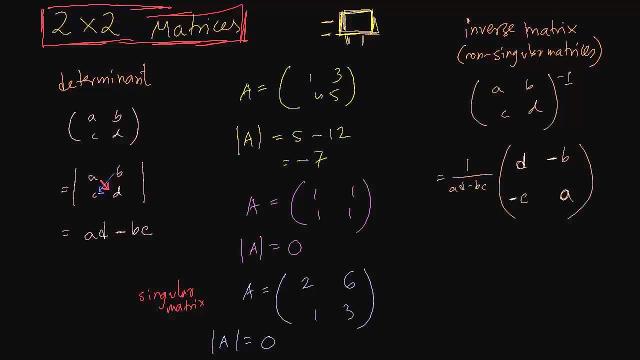 And you make it minus C. So that's how you find the inverse of a matrix. So an example would be: Suppose you have a matrix A Which is 1,, 2,, 3,, 4. And you want to find the inverse of this matrix. 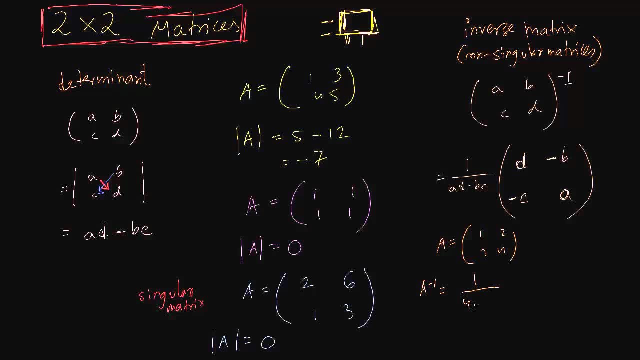 So this is going to be 1 divided by 4.. 1 is 4. Minus 3 is 6.. And then we can just change the position here. So this is going to be 4 over here. This is going to be 1 over here. 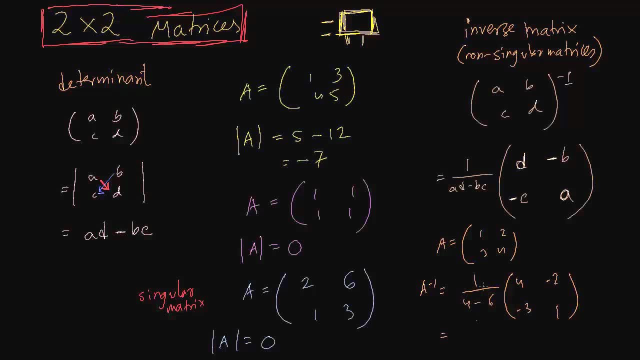 And this is going to be minus 2.. And this is going to be minus 3.. You can keep it like this Or you can do the scalar multiplication. Remember this is a constant 1 by minus 2.. So minus half. 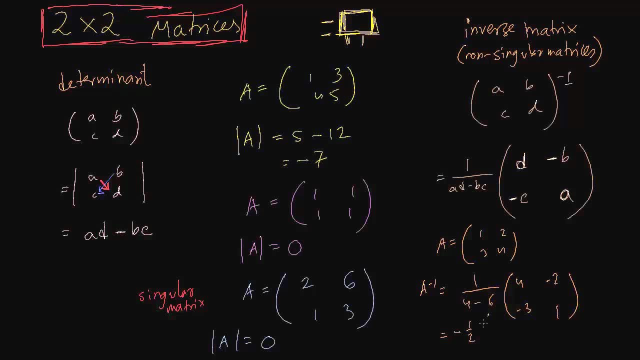 So if I write here minus half And multiply it with that, Okay. So that would mean I'm going to multiply minus half with 4. Minus half with minus 2.. Then minus half with minus 3.. And minus half with 1.. 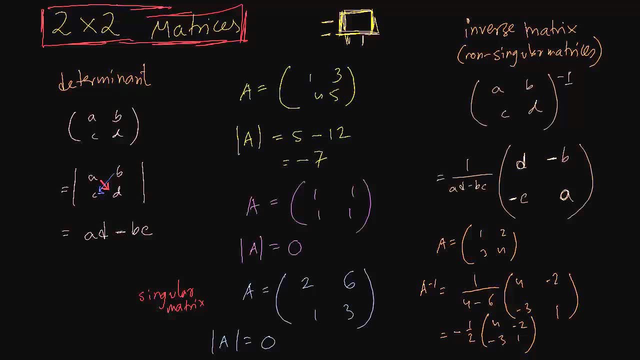 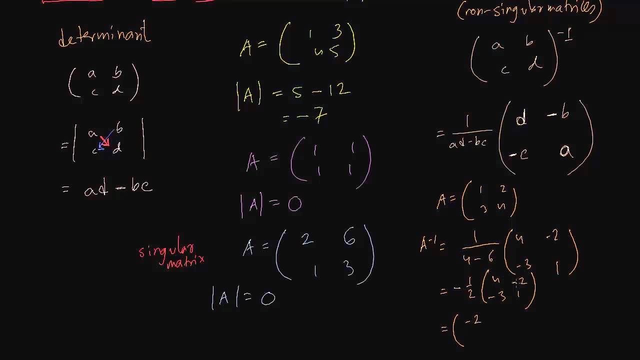 So this is what it looks like. Okay, So what we have here is: Minus half with 4 is minus 2.. Minus half with minus 2 is 1.. Minus half with minus 3 is 3 by 2.. 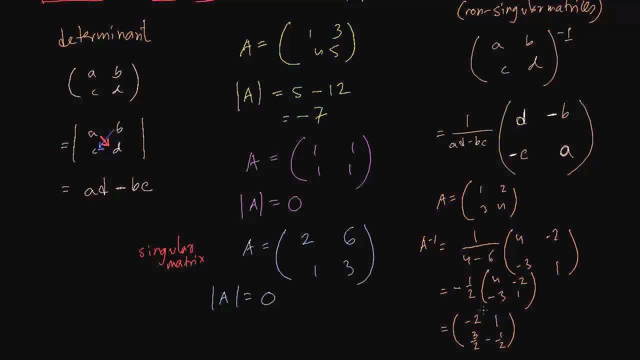 And minus half with 1 is minus half, So that's an inverse of a matrix. There is a special rule worth remembering: If you multiply the inverse of a matrix with itself, You end up with a special 2 by 2 matrix called the identity matrix. 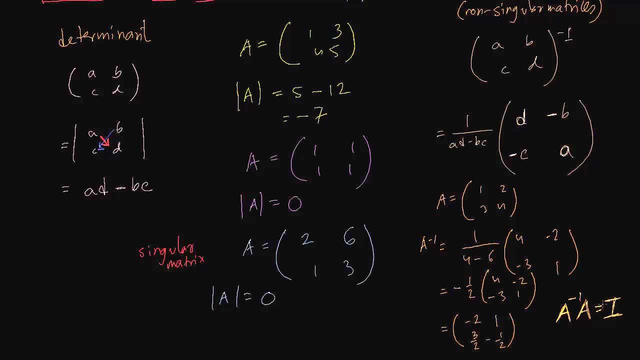 An identity matrix is a matrix with 1's and 0's, So this particular identity matrix is: The diagonals are 1.. So that's the special case. When you have the inverse of a matrix multiplied by the matrix itself, You have a special matrix. 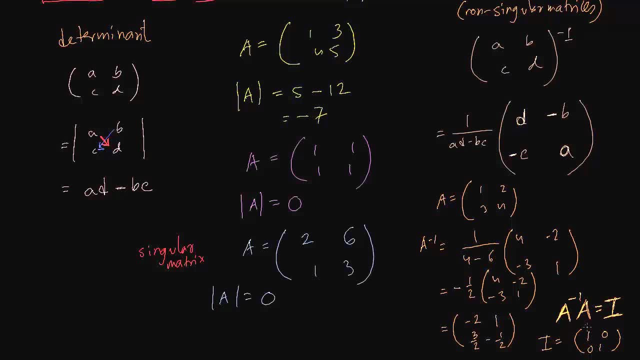 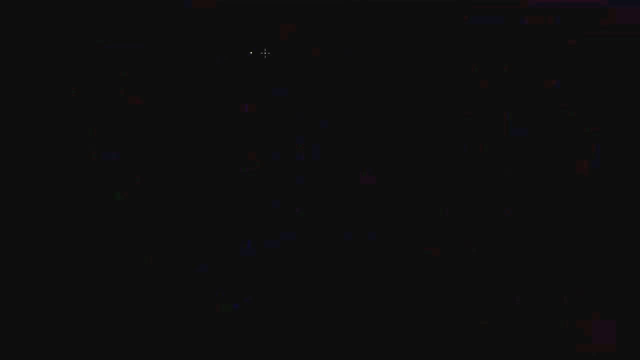 It's called an identity matrix. It's a particularly a 2 by 2 matrix, in this case, With diagonals as 1's and the rest as 0's, So these things are worth remembering. So, when you are remembering matrices, 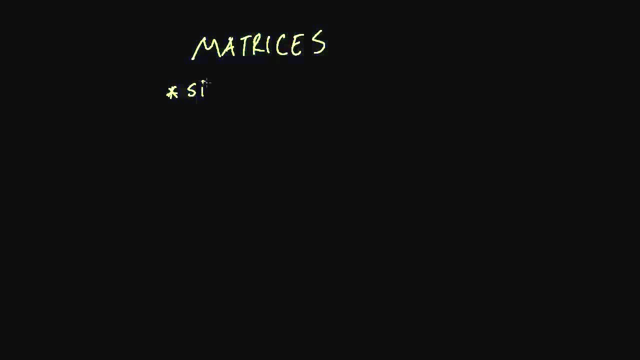 Matrices. First thing, What is the size of a matrix? The size of a matrix is The number of rows times the number of columns. Next The addition- Subtraction. So how do you add or subtract the matrices? Remember? 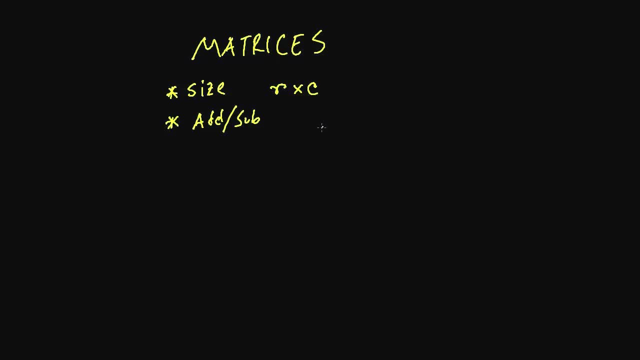 You just add the same positions And basic addition and basic subtraction, And the two sides of the matrices has to be the same. The first one is A by B. The second one also has to be A by B. That has to be the same. 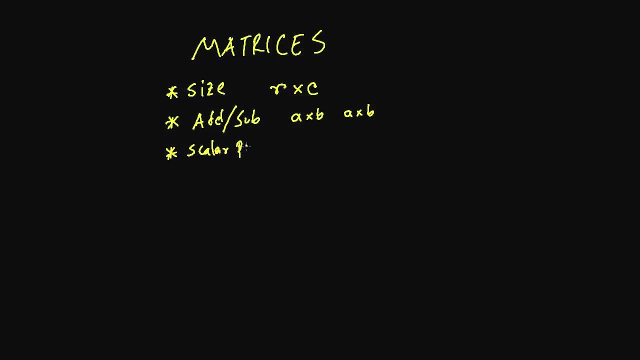 Next We have the scalar product of matrices. Scalar product. Here the size of the matrix doesn't matter. You just multiply the matrix with a number. Then we have the multiplication. How do you multiply matrices? This is a bit difficult. It has a special rule. 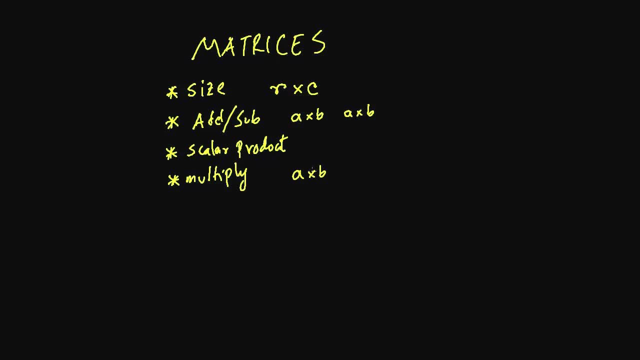 And the size. You cannot multiply every matrix with another matrix. It is not allowed. You have to make sure the column of the first matrix is the same as the row of the second matrix And the resulting matrix will have a size of A by C. 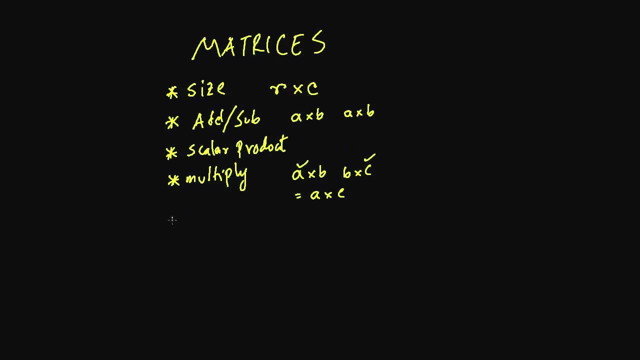 This A by C. The next thing is some special rule for square matrices, In this particular case, 2 by 2 square matrices. So here we have the determinant of a matrix, Then we have the concept of the determinant being 0 or a singular matrix. 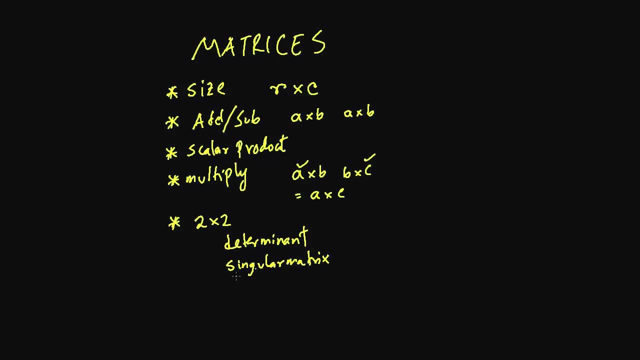 Singular matrix, Which simply means that the determinant is 0. Then we have inverse of a matrix. One more thing needs to be mentioned before I end this. It is solving equations using matrices. So solving equations or system of linear equations, If we have an equation like 3x plus y equals to 2.. 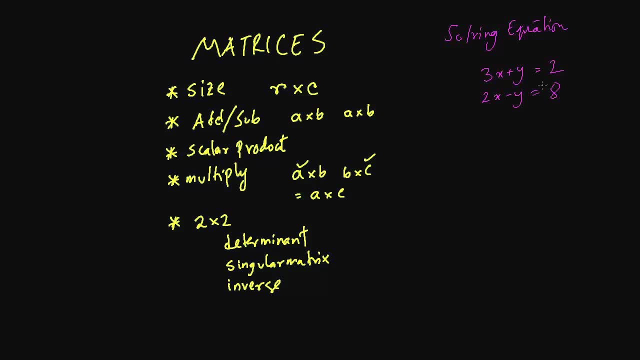 And 2x minus y equals to 8.. By the method of elimination We would solve it like this: We would cancel off y And when we add this It would be like: 3x plus 2x is 5x. 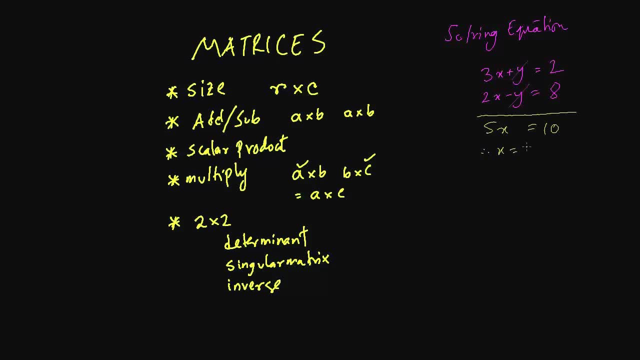 8 plus 2 is 10.. Divided by x equals to 2.. 10 divided by 5 is 2.. And when we put the value of 2 in one of the equations, It turns out to be 3 into 2 plus y. 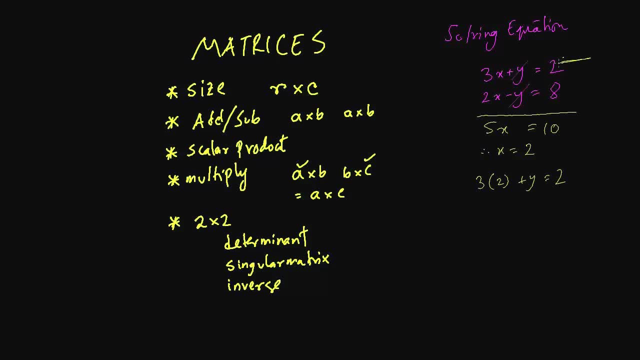 Equals to 2.. I am putting it in the first equation here, Right over here, So that turns out to be: y equals to 3 into 2 is 6.. I keep saying 3. I don't know why. 3 times 2 is 6.. 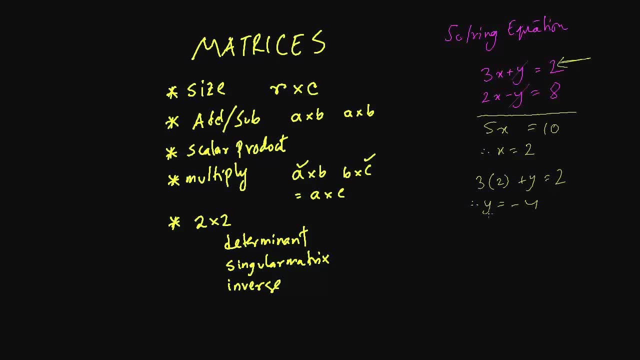 So y equals to 2 minus 6 is minus 4.. So we find the solution of the equation to be: x equals to 2 and y equals to minus 4.. Now let's see whether the same thing can be done using matrices. 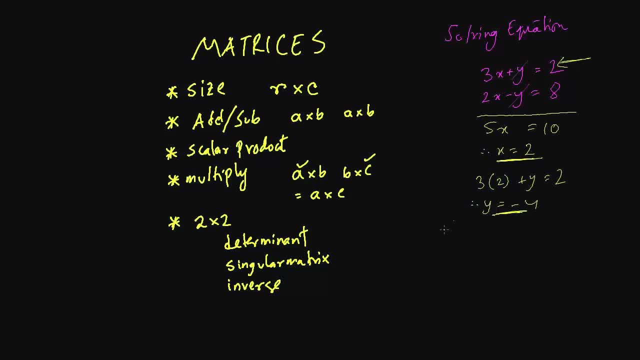 But this is the trick: We write the coefficient of x and y into a matrix. So the coefficient of x is 3.. The coefficient of y is 1.. The coefficient of x, here in the second row, is 2.. And here is minus 1.. 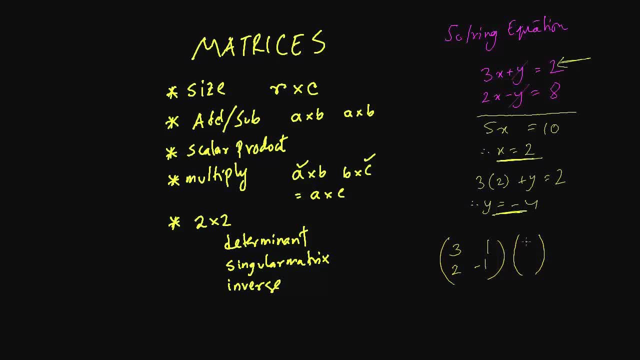 Then we multiply it with the variables x and y. x, y Equals to. We write down the values in the other matrix, 2, 8.. Now this: When we have a matrix with only one column, We call it a column vector. 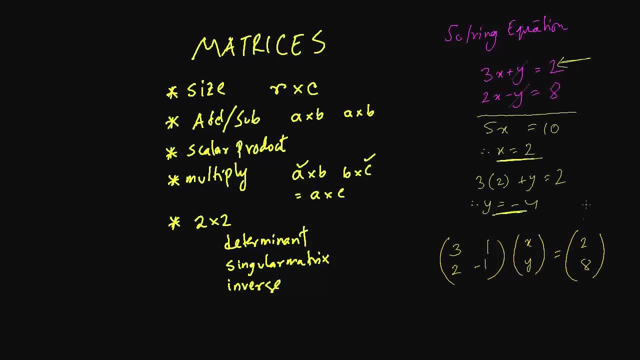 I will talk a little bit about this later on. So this is column vector. We have one column, So let's, I am going to use the inverse for this. So we write Therefore: Remember, in matrix we don't have any division. 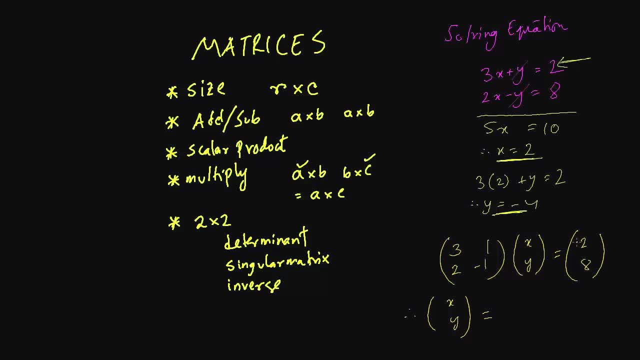 We use inverse, So we take this to the other side And always remember we write it at front, Not after 2, 8.. This column vector In front of the column vector, Column vector again, is a matrix with only one column. 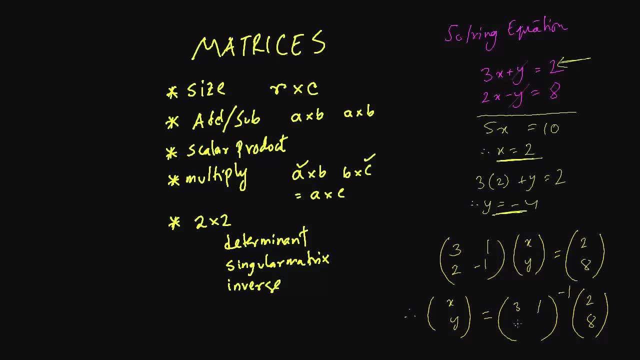 So this is going to be 3, 1.. 2 minus 1.. The inverse of this- And remember inverse- we write it as Minus 1.. We don't write the inverse as 1 divided by a. 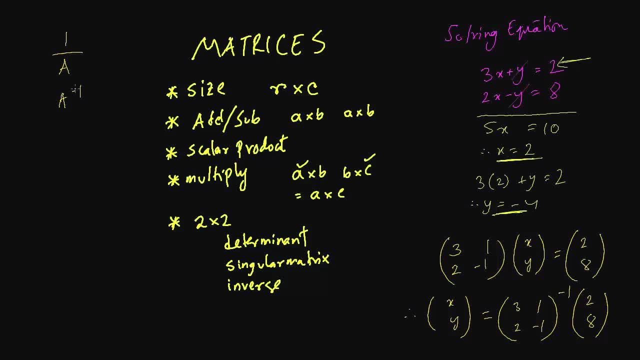 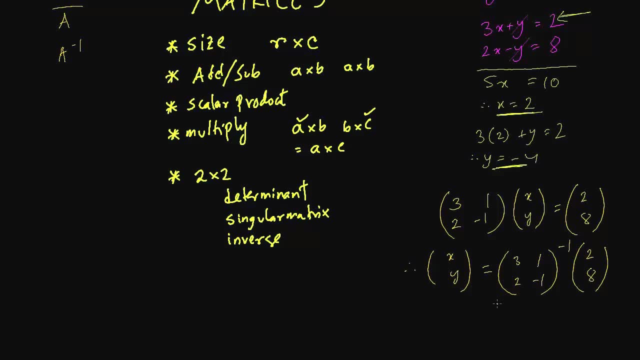 Unfortunately, we don't write that. We write a to the power minus 1.. So now we can move on. Let's find the inverse of this matrix. I don't think I am going to have space over here, So let me come right over here and do it. 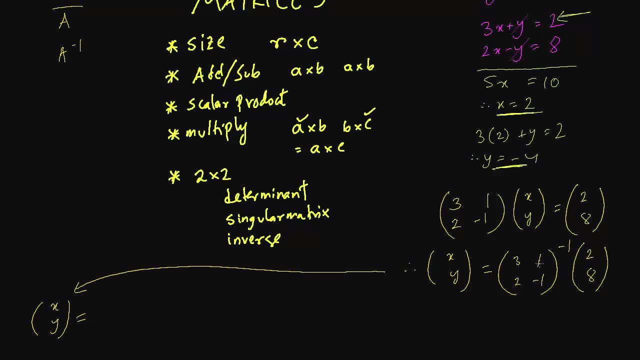 So x, y. So the inverse of this matrix is going to be 1 by determinant, Which is AD minus BC. So which is 3 into minus 1 is minus 3.. Minus 1 into 2 is 2.. 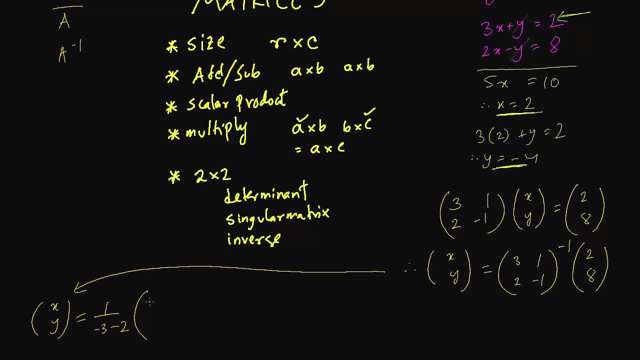 So, and we are going to change the positions here For the inverse, this is going to be minus 1, 3.. And we are going to change the sign over here, Which is going to be minus 1, minus 2.. We found the inverse. 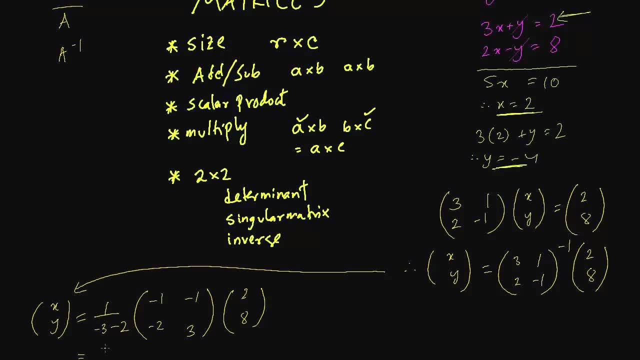 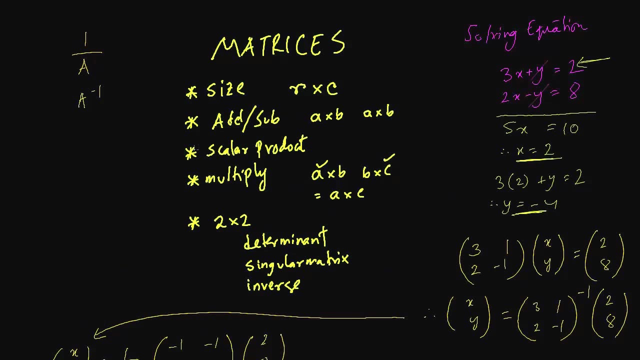 Now we have to multiply this. I am going to keep the determinant over here, Which is 1, by minus 6.. Minus 5 over here, Okay. So now let's multiply these two, So we have: Okay, this is better. 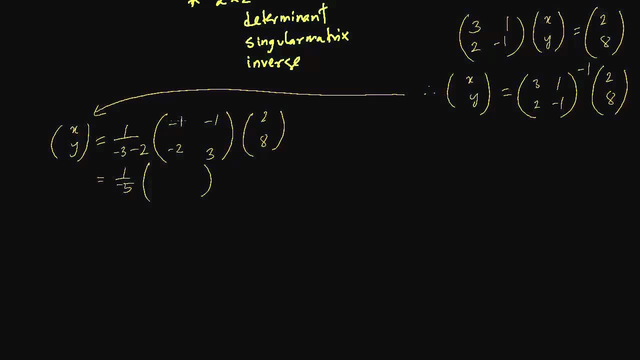 So we have, We have to multiply this row with this column. Remember, we multiply this row with this column, So let me mark here: So this row With this column over here Is going to be minus 1.. Times 2 is minus 2.. 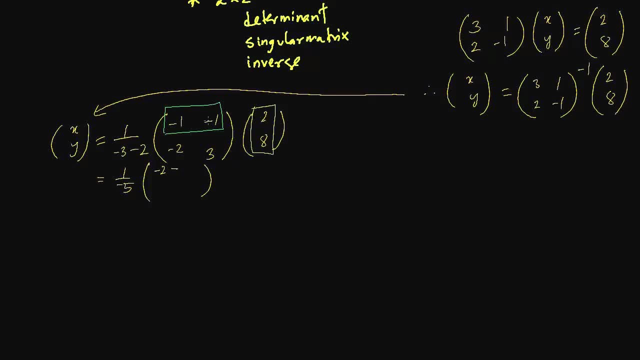 Then we have Minus. Since it is minus, I am going to write minus instead of plus. Minus 1 into 8 is minus 8.. Then we move on to the next row And do the same thing over here. 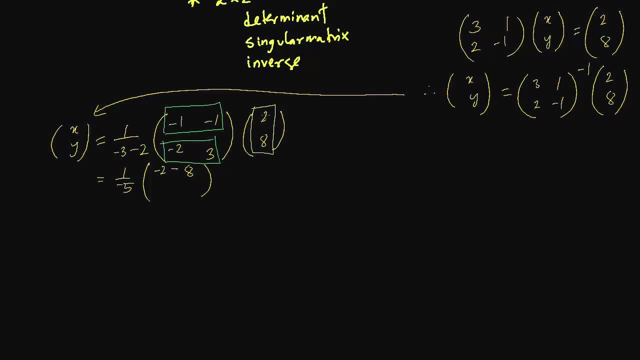 So this is going to be Minus. 2 into 2 is minus 4.. And 3 into 8 is going to be 24.. So let's see how this turns out to be. This is minus 10.. And this is going to be 24. minus 4 is 20.. 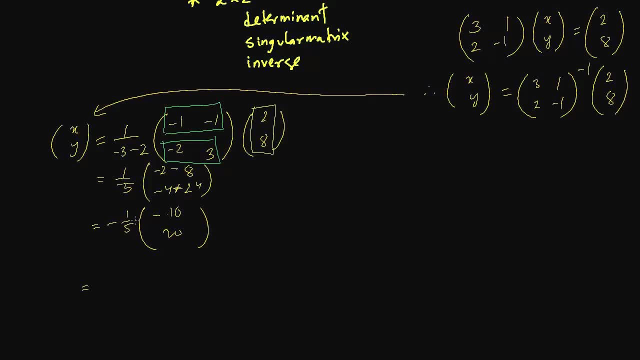 So if I multiply this scalar product now, It is much easier to do it now at the end Rather than at the beginning. So minus 1 by 5 into minus 10 is 2.. Minus 1 by 5 multiplied by 20 is minus 4.. 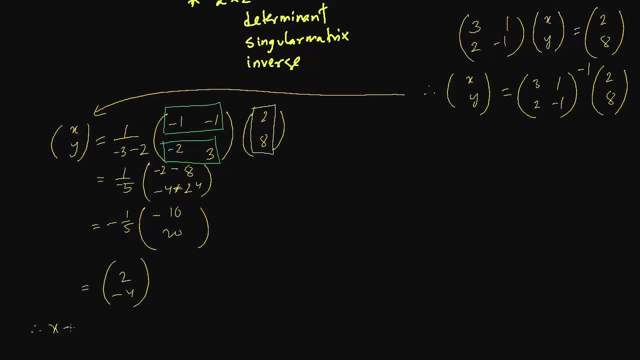 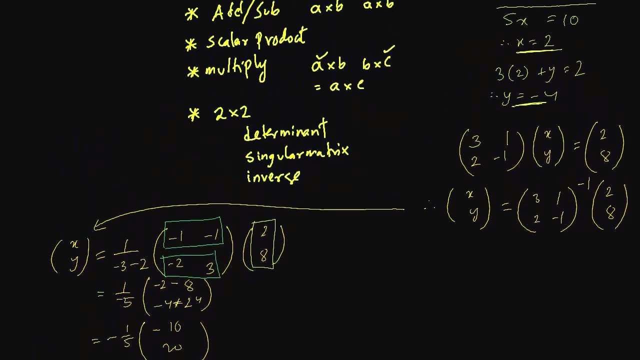 So this is equals to xy. So therefore, x equals to 2. And y equals to minus 4.. So let's check the elimination method that we got. We got 2 and minus 4.. We got 2 and minus 4.. 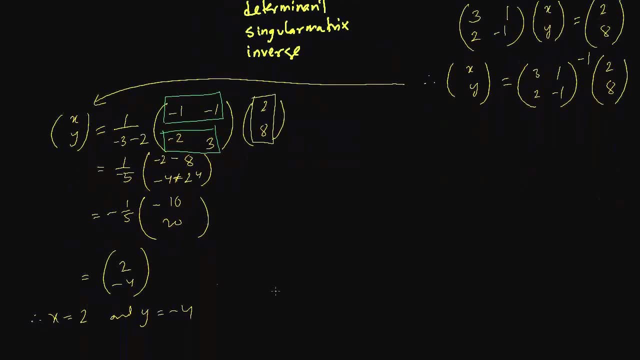 Exactly what we got over here. Now let me talk a little bit about column vectors: Column vectors. For column vectors, you need a little bit background about vectors, So let me tell you: Vectors are represented with a line. Vector is a line with an arrow. 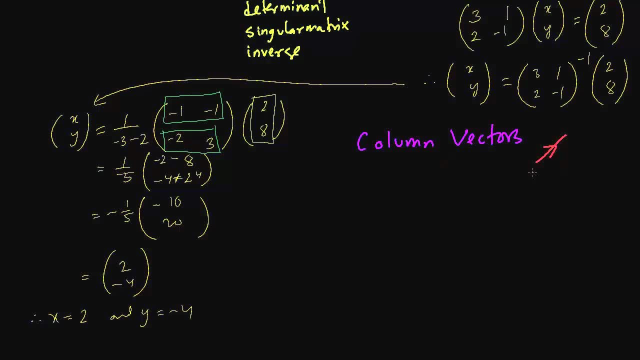 And they are usually written as Suppose: if you have a point here a And if you have a point here o, So the vector would be called The position. vector of a is oa, And it is often written with ij or ab. So suppose it is written as xi plus yj. 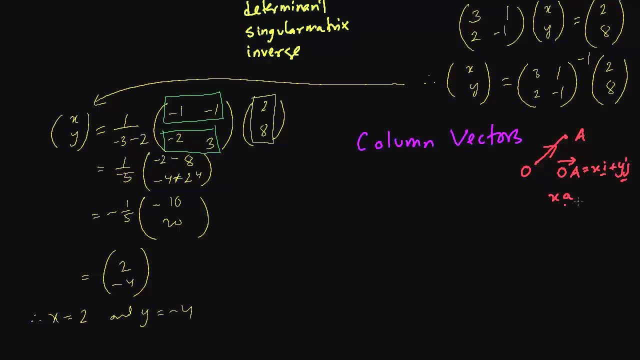 Or it can also be written as xa plus yb, Where a contains the xy material And b contains the ij material. So it is called ij materials. Now if you have a point xy And suppose that point is a, You can also express the vector oa in the column vector format. 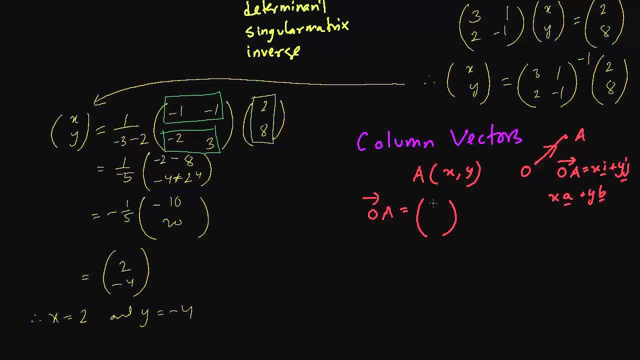 And it is written with a matrix that has only one column. That's called a column vector, So it is a matrix with one column. So what can we do with this? The first thing we can do is we can find the length of this line. 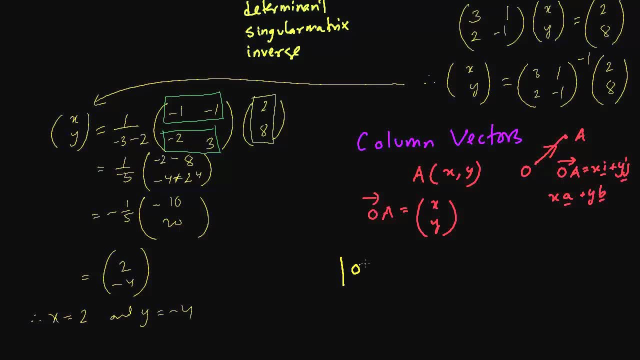 So the length of this line, Written as these two bars, Not determinant. this time It is called the modulus of the vector, Or the length of a line of a vector. So we write it using the Pythagorean theorem: Square root of x squared plus y squared. 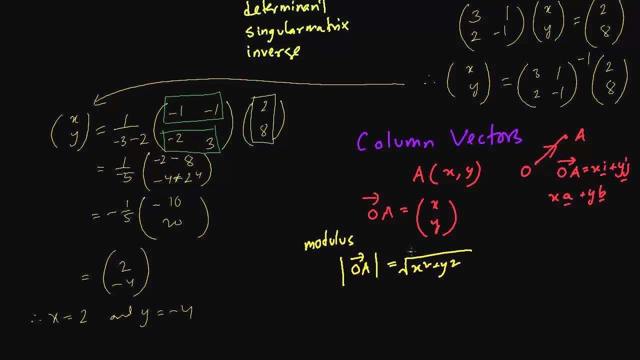 So that's the modulus of a column vector, Which is a matrix, really A matrix with one column. Another thing that we can do here, Using matrices and using vectors, Is that when you have two vectors- Let me write this down- Suppose you have a column vector. 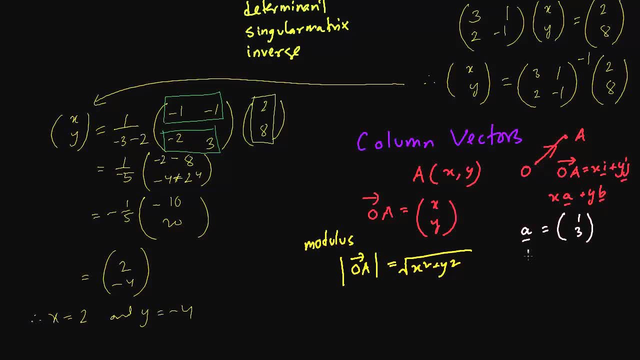 1, 3.. And you have another column vector, 5, 7.. And you are asked to find the modulus of a plus b. So what you do? You first find out the value of a plus b. So a plus b is going to be the addition of the column vectors. 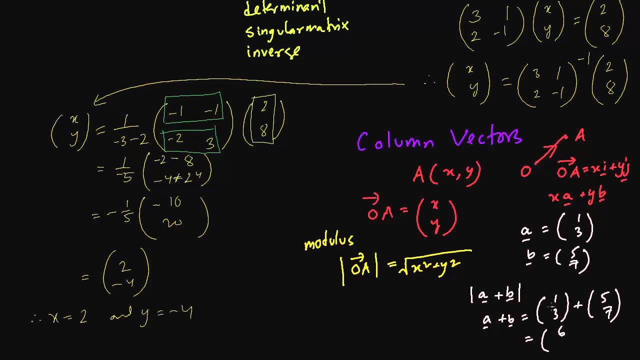 And you are going to get: 1 plus 5 is 6.. 3 plus 7 is 10.. Once you know this, Now you can find the modulus of the column vector Which is going to be square root of the first row squared. 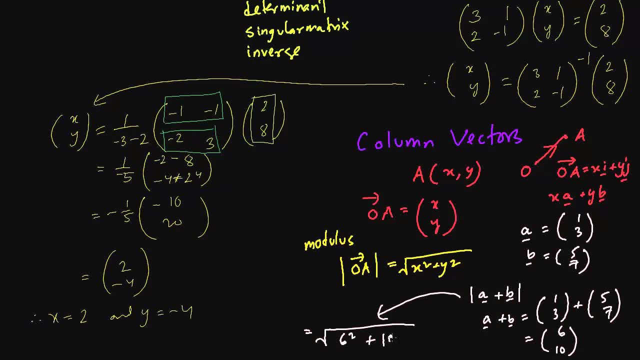 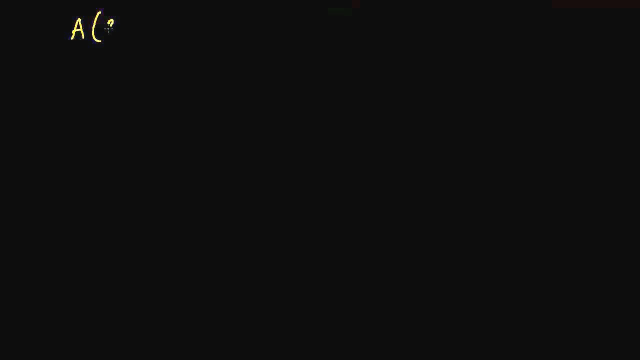 Plus the second one squared, So this is going to be 100 plus 36.. Square root of 136.. Let me just do one more example before I end this. Okay, So suppose you have a point A And it is 3, 5.. 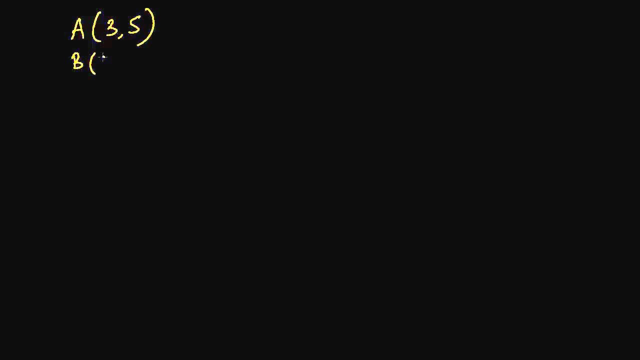 You have a point B, Which is 4, 7.. Now, if I want to write this as column vector, That means the position vector. Remember, it's point A from the origin And this is point B from the origin. So you write the position vector as 3, 5.. 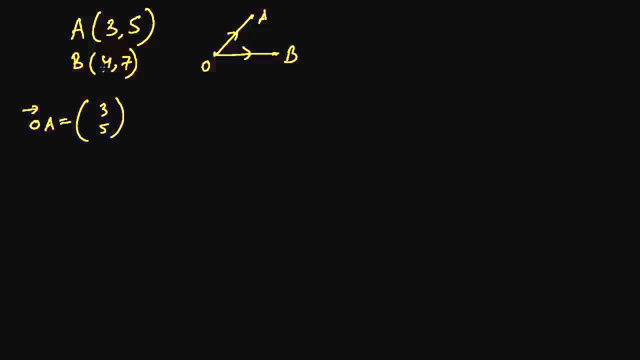 Which is matrix with one column or column vector, And the position vector Of B is going to be 4, 7.. So that's that. Now I'm going to ask you Find the vector AB. Now there is a position vector rule. 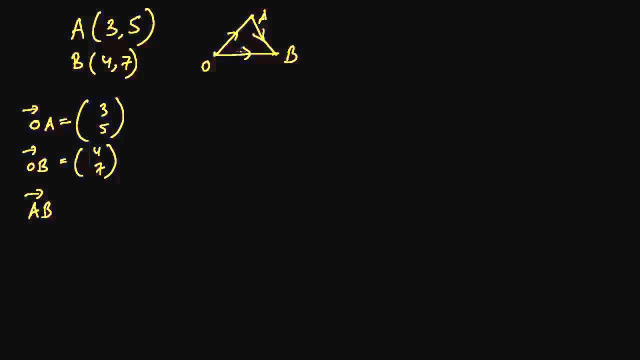 The vector AB. We can use the triangle rule Or we can use the position vector rule. The position vector rule says that One vector is the difference of the final vector. So if this is AB, This point is known as the terminal point. 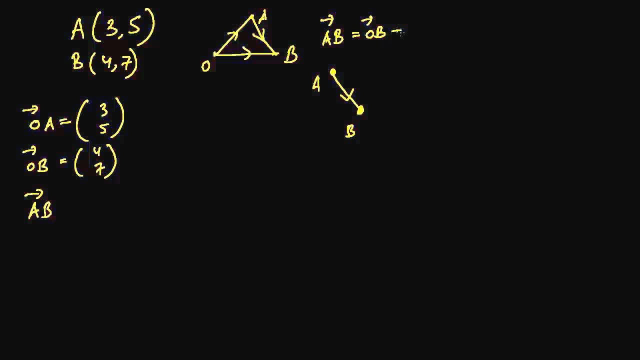 This is known as the initial point, The position vector of the terminal point Subtract the position vector of the initial point, So that means We are going to do the column vector 4, 7.. Minus 3, 5.. 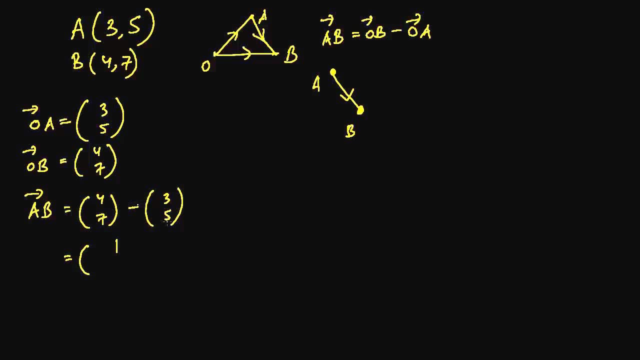 And it turns out to be: 4 minus 3 is 1.. 7 minus 5 is 2.. So that's it. Now the question is: Find the modulus vector, Modulus of the vector, Which means AB modulus. 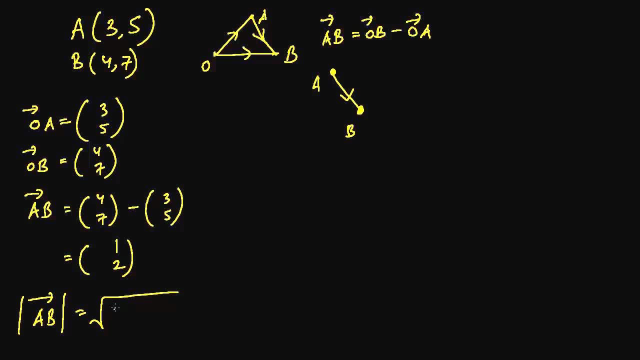 Equals to square root of This row squared, So 1 squared Plus this Square, Which is going to be Square root of 1. Plus 4., Which is square root of 5.. Now, Since this is the length of a line, 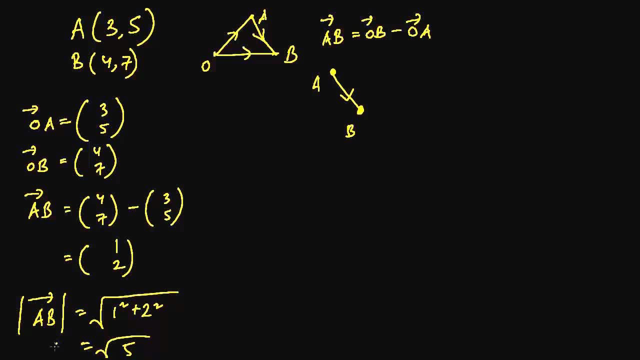 We can also write Modulus of vector AB As simply AB Length of the line. 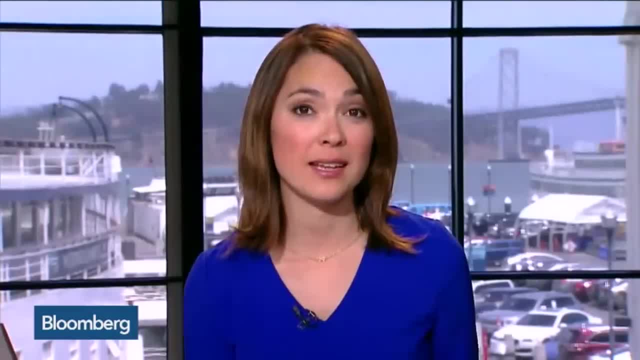 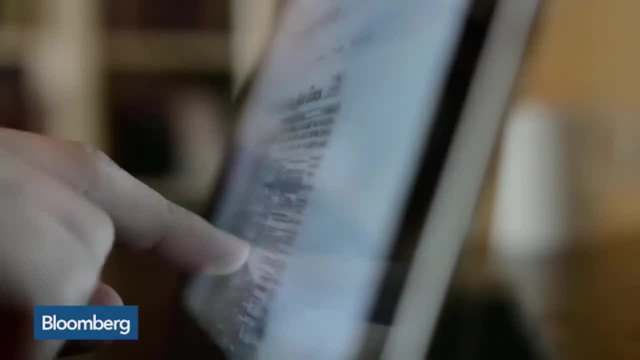 It is time now for the Daily Byte, one number that tells a whole lot Today: 14 gigabytes, That is the amount of mobile data the average North American smartphone user is expected to use every month by 2020.. This according to an Ericsson Mobility report. 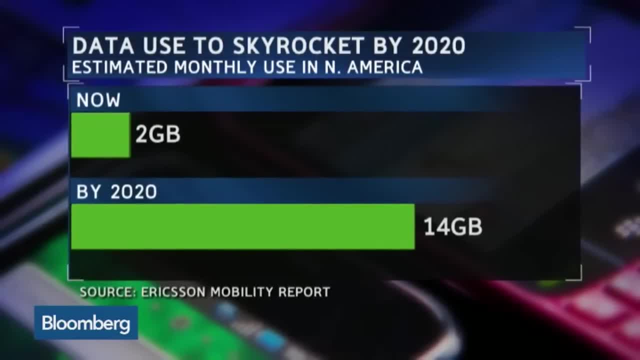 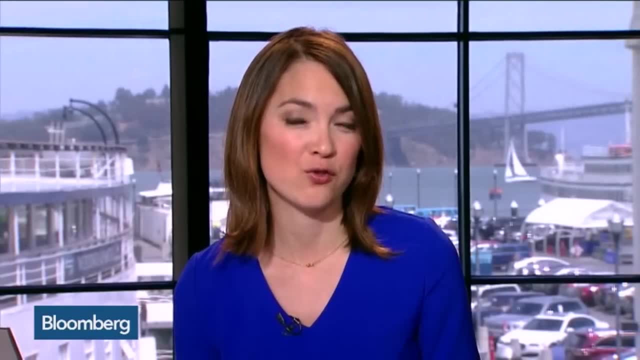 That is a massive six-fold increase from today's norm of about 2.4 gigs a month. So what could we possibly be doing with that much data? We crunched the numbers: You'd have to stream 117 episodes of Bloomberg West to hit 14 gigs of mobile data use. 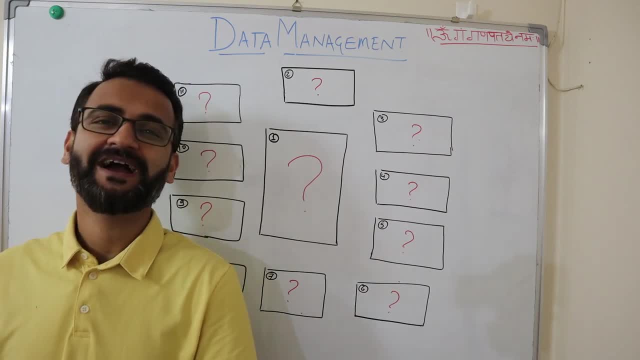 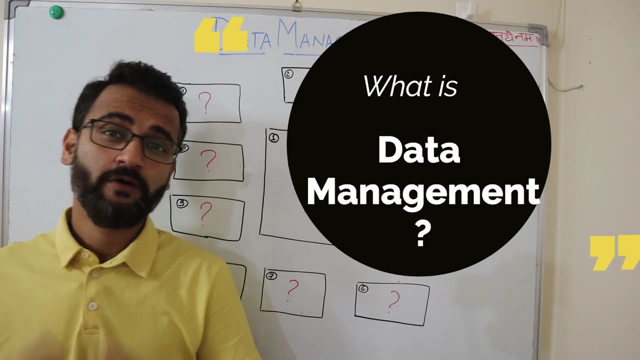 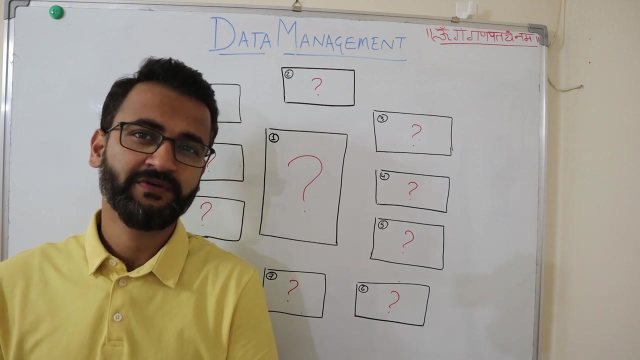 Hello friends, welcome to ITK Funday, your own channel, where we make IT interesting for everyone, And in this video we will understand what is data management. Now, when we say data management, it pretty much covers every aspect of data and overall data industry in which we work.